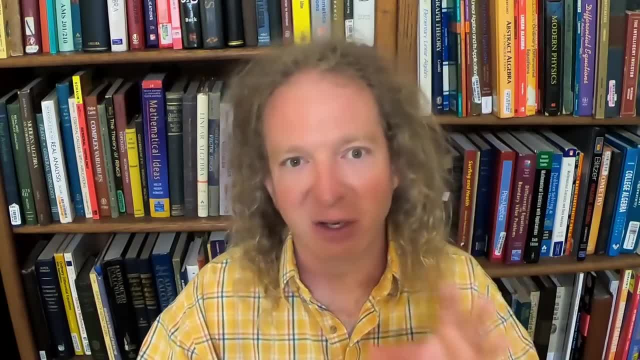 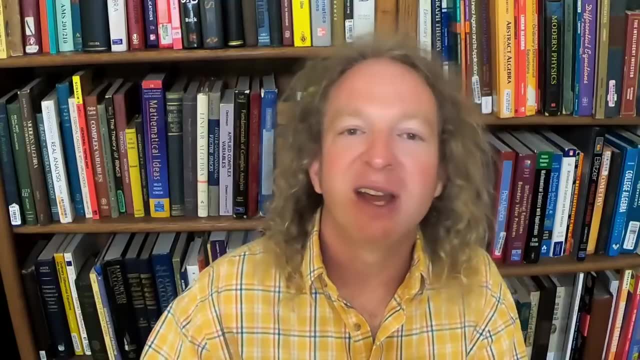 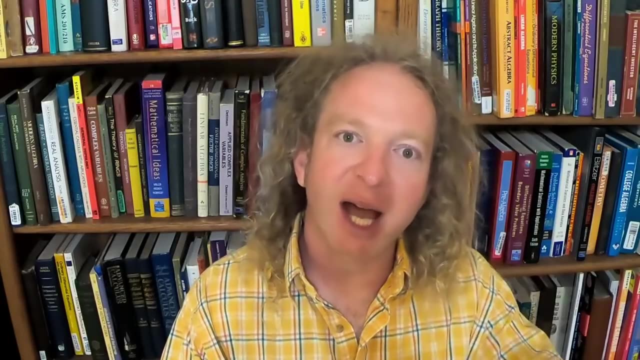 over all of your notes. if you're watching videos and you're taking, like, an online class, make notes from the videos. so as you watch the videos, pause the video and write stuff down. that is the beauty of online classes. that is the beauty of videos. right, because if you're taking a class and it's in person, a lot 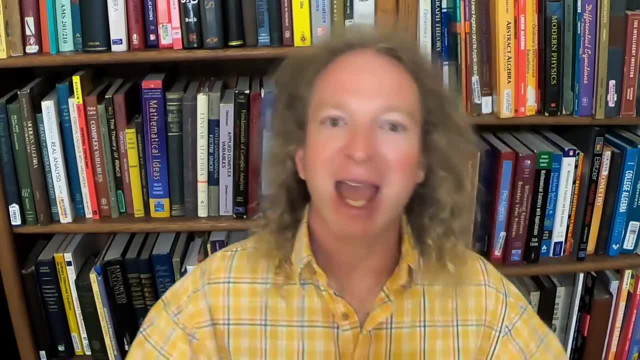 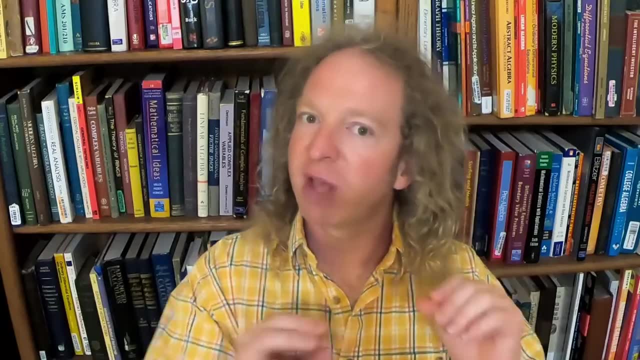 of times it's really hard to to write down everything the teacher says and pay attention. at the same time. I know people who who just sit there and they don't take notes and they say they have a picture memory. that's great for those people. I'm not one of those people. I'm a 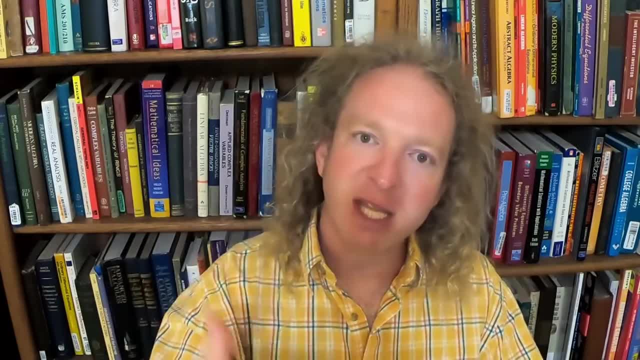 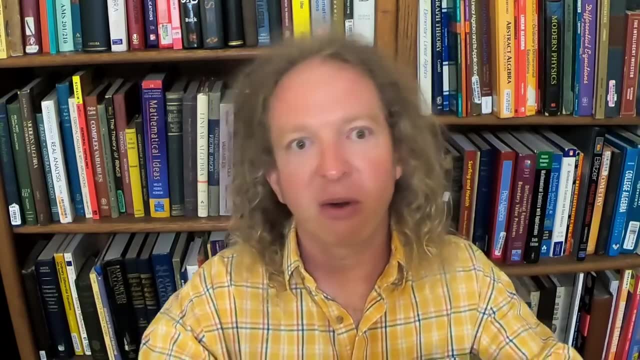 notary public loan signing agent: taker right. I have to go back and I have to read it many, many, many times in order to fully understand it. most of the time when I watch a video like a lecture video, or if I go to a classroom and watch an actual lecture in a classroom, I 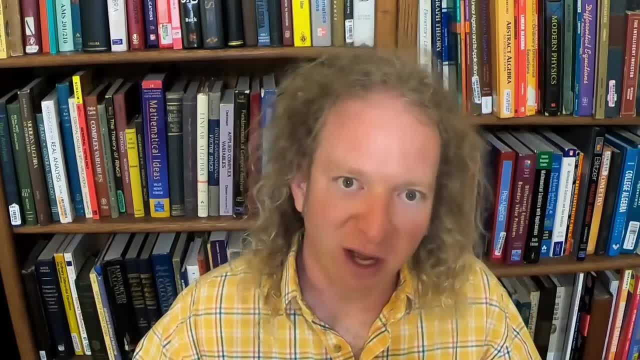 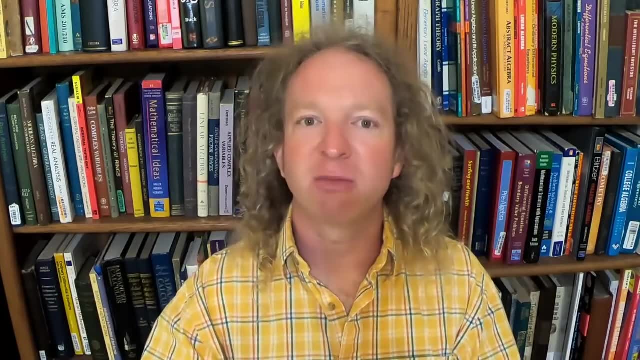 understood. maybe 60 to 70% was being taught. that's it. 60 to 70% of what was being taught is what I understood. so I'm not one of those people who has a picture memory. so note-taking was always critical and then going over those notes. 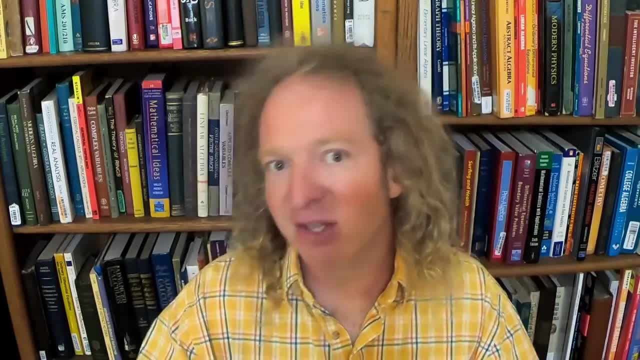 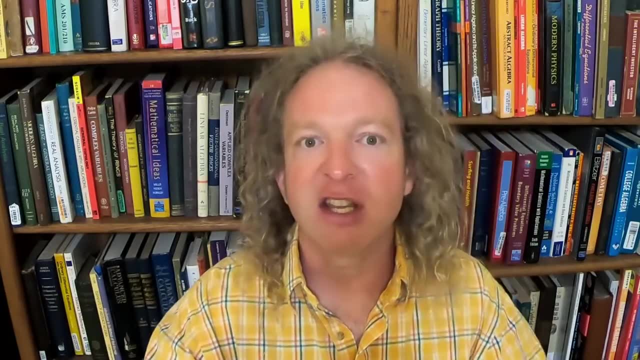 is super, super key. so again, if you're taking a live class, just write down as much as you can and then, when you get home, just make sure to dissect those notes and go through them line by line, rewrite them in a neater fashion so you have them in a place that you can access them, and also the act of like writing. 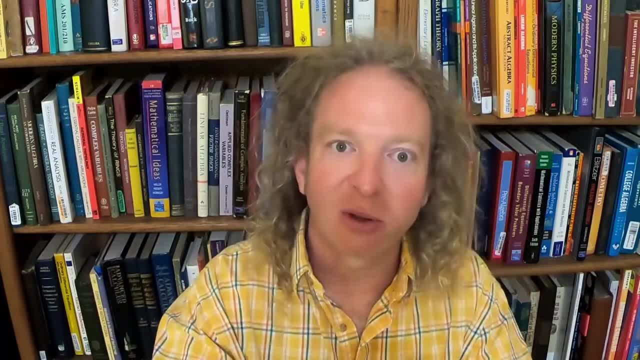 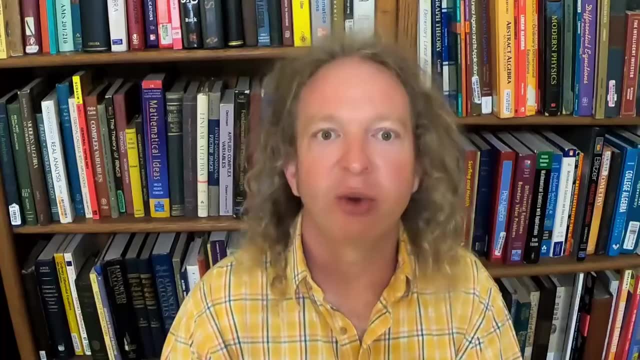 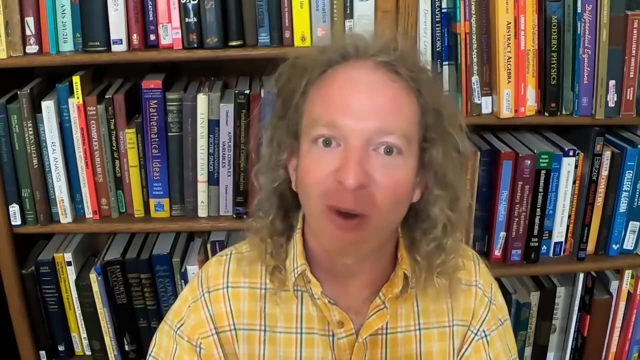 down on a piece of paper, writing down everything that you learn. just writing it again makes you learn right. it's not just about like sitting down and and watching a video or listening to a lecture and absorbing it. no, no, no. if it was that easy, everyone would do it right and you know you wouldn't be watching this video. 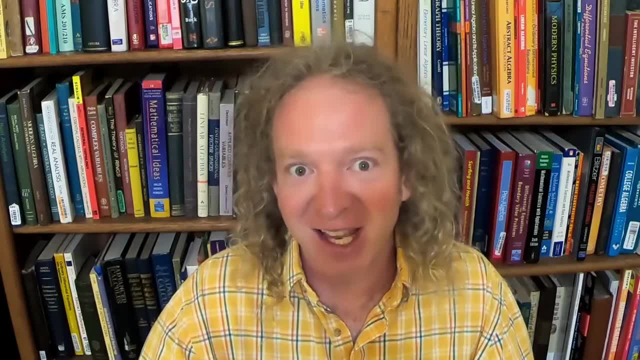 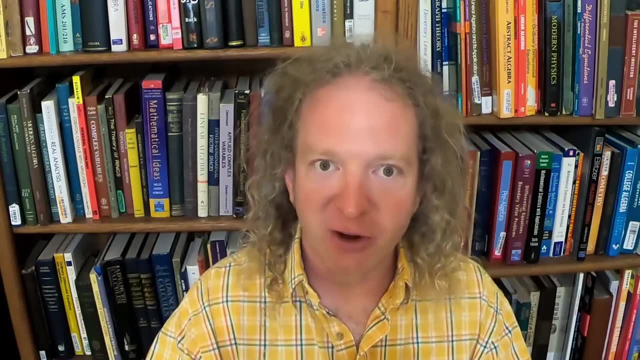 everyone would just like: oh yeah, that makes sense, and they would just get an A in calculus. it doesn't work that way. right, by writing it down again, it is extremely, extremely beneficial. also, just for emphasis, if it's an online class and you're watching videos, make notes of the videos, pause the video, rewind it, watch. 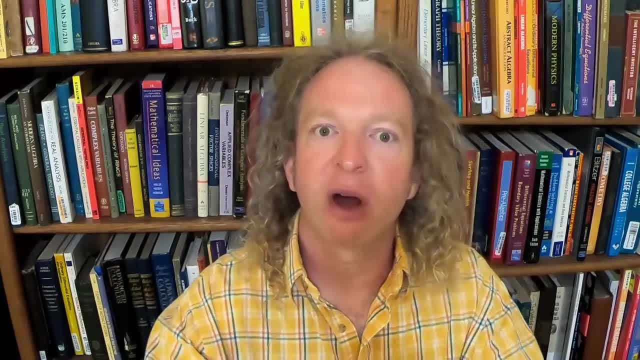 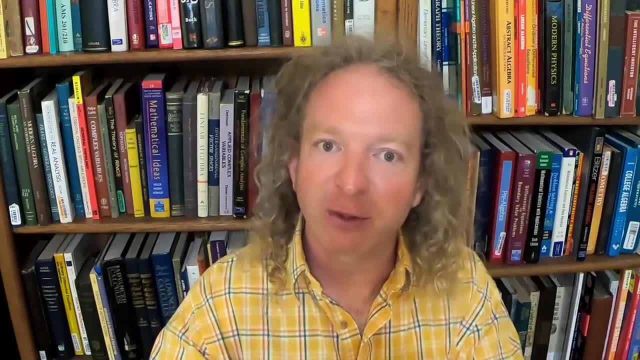 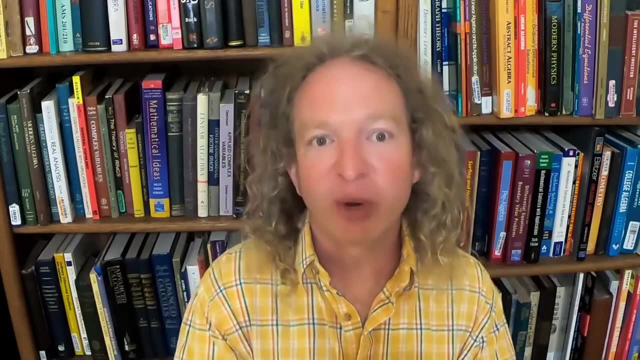 if you actually do that, if you can actually redo all of the examples from class, usually that's enough to get a really really, really good grade, even even an A. the third thing that you should do is to actually redo the homework now. this seems completely insane, I think, to a lot of people, to me. 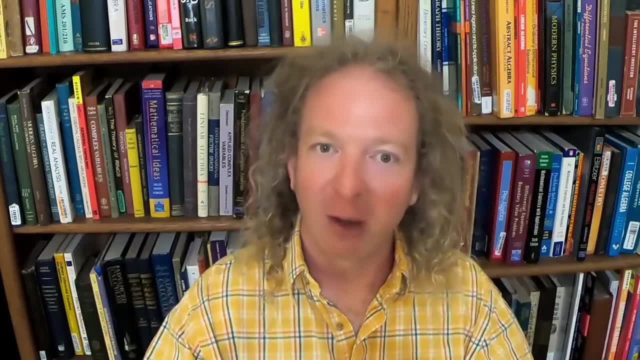 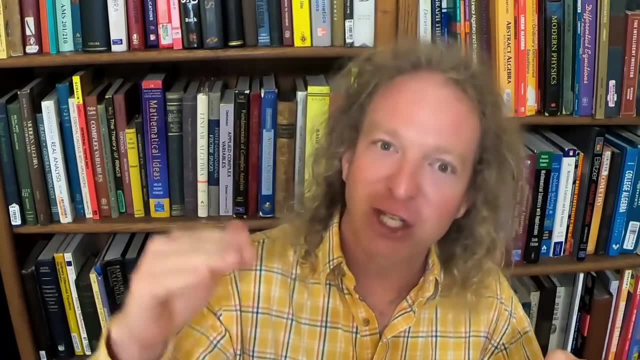 it does not. I am an overdoer, right, I wouldn't. I don't want to say over achievers, because I don't think I'm that, but I totally tend to overdo it. whether I overachieve, I don't know. maybe achieve to some extent, but not, not an. 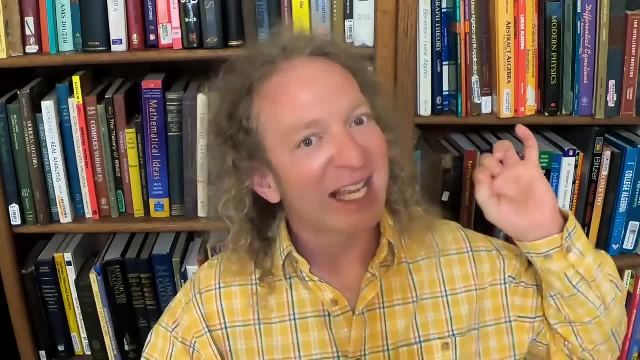 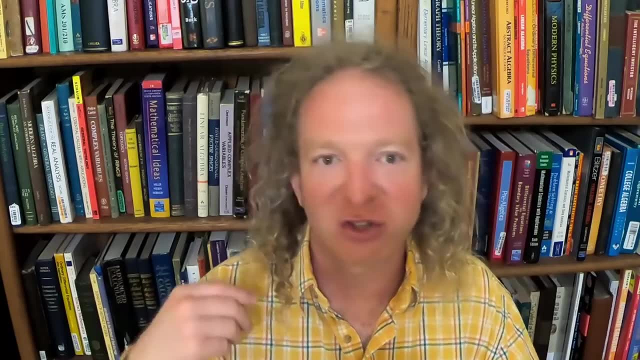 overachiever, overdoer. so I would study excessively. I would do all of the homework and then just redo it right, just do it again, just randomly pick problems and then just do them. I know this seems excessive and it takes a lot of time, but if you want to get an A, 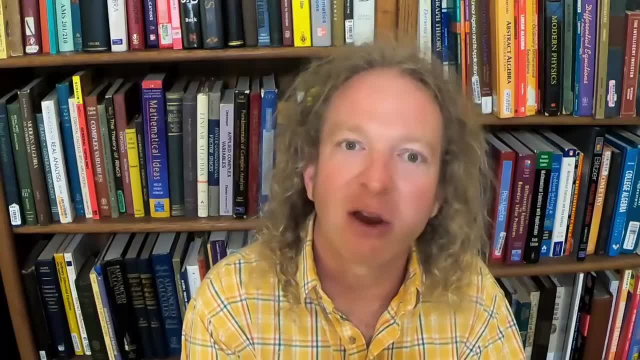 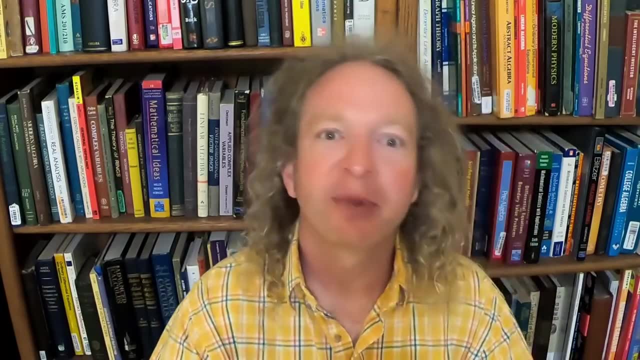 in your class, you know. think about how much, how much it means to you. right? are you willing to make that sacrifice? you're willing to, you know. do all of the homework, go over all of your notes and then redo the homework. trust me, it is totally worth it. the fourth thing you should do is to 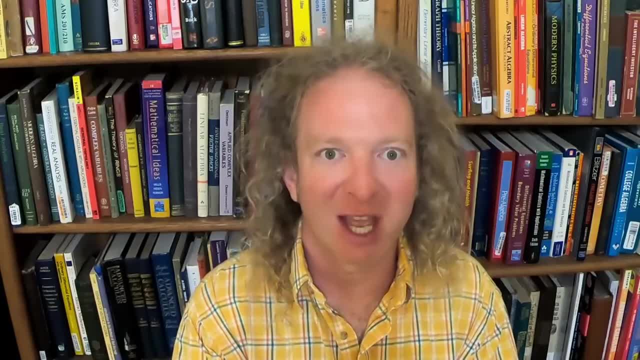 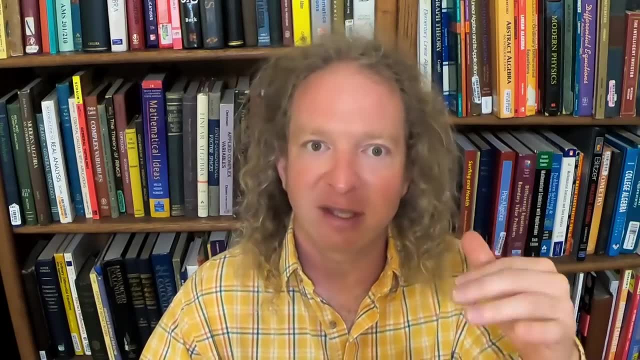 actually pay attention to the topic list for the exam. okay, so hopefully, if you're taking a class, your teacher has told you you know what to study like. hey, make sure you go over this, this, this and this. what I do- because I teach now- is in my 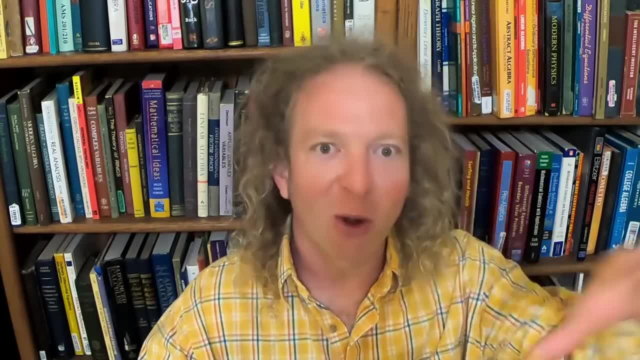 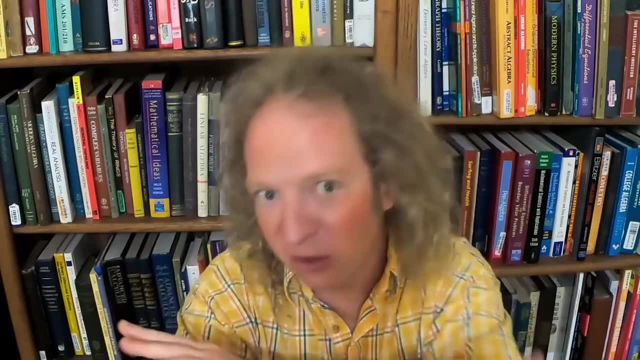 face-to-face classes. I do like an in-class review and I go over all of the topics in my online classes. I give them a list of topics and if they do the homework in those topics, they will get like they can get an A guaranteed. now. everyone is different, right? every teacher is different. every teacher is. 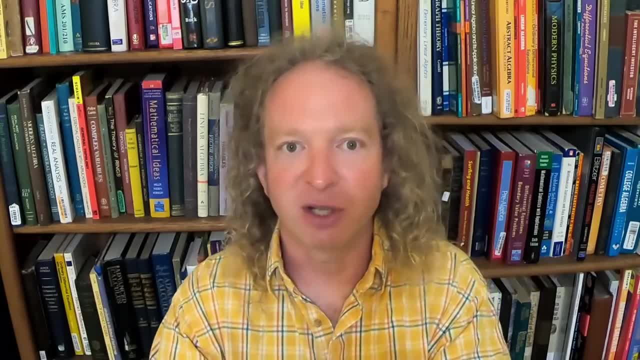 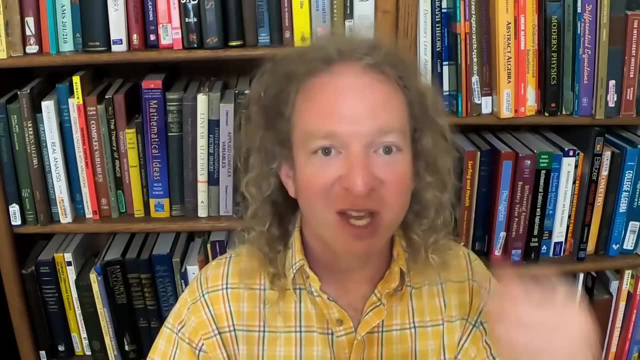 different. so what you will see on a test will vary from teacher to teacher. the worst situation is you know your teacher says, hey, you know, go over topics XYZ, and then you take the test and it's something completely different. that is the absolute worst case scenario. so if that happens, you have a fallback plan. 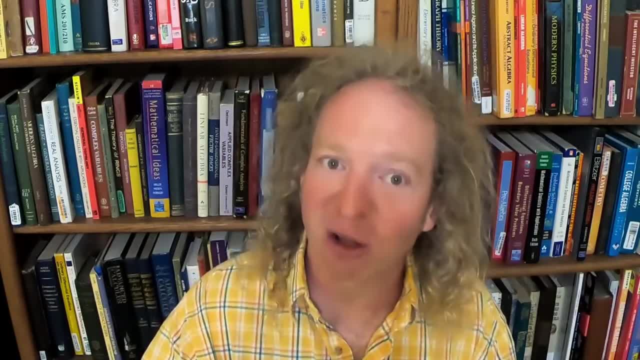 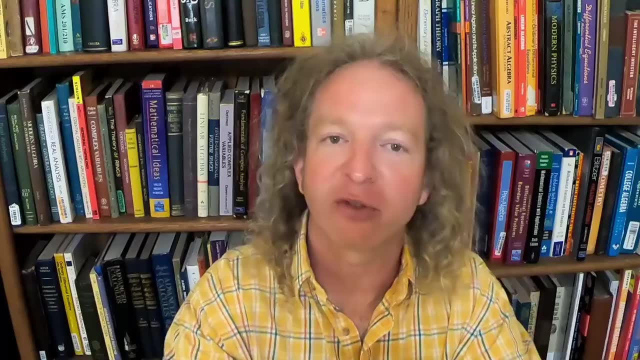 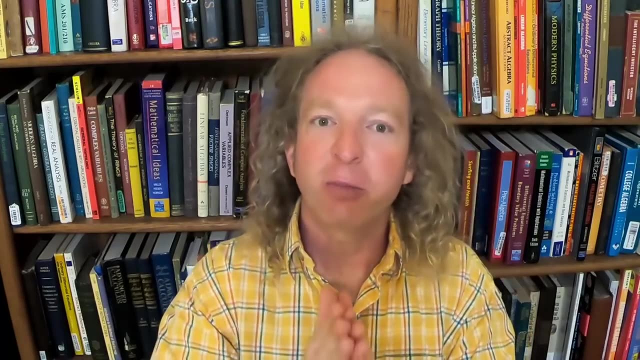 right, you're doing all of the homework. you're redoing all of the homework already and you're redoing all of the videos or lecture note examples- right, you're redoing all of your notes. so, in theory, because you're doing that on top of going over a topic list, if you have one, then you're pretty much guaranteed. 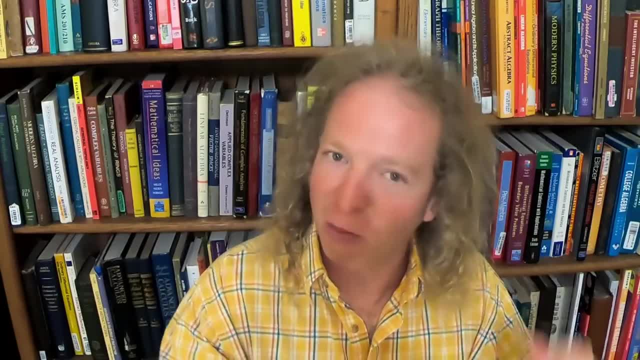 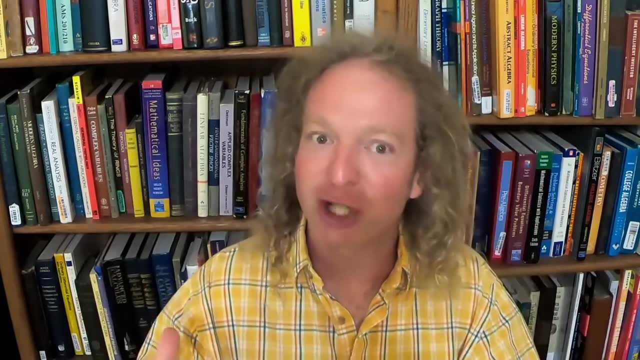 to get a good grade, you're going to do better. if you do that much, you're probably gonna get an A, trust me. okay, like I've taken a lot of math classes- I'm not saying I'm like some super genius, but I have taken a lot of- 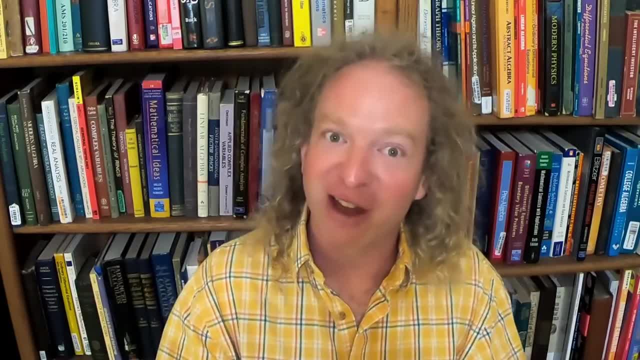 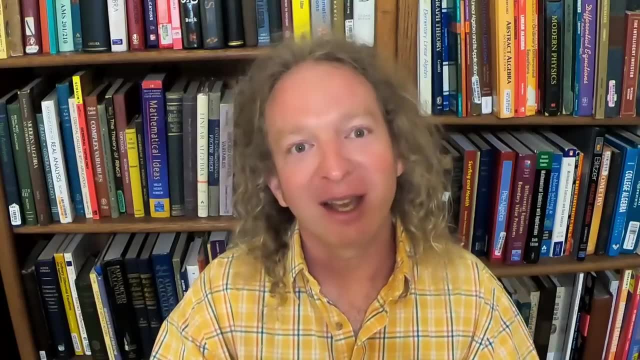 classes and I have gotten, you know, a lot of A's and I've taken a lot of tests. I feel like I'm a professional test taker at this point. is that a good life skill? does thereückt they maybe- well, probably not- more of a certified math? 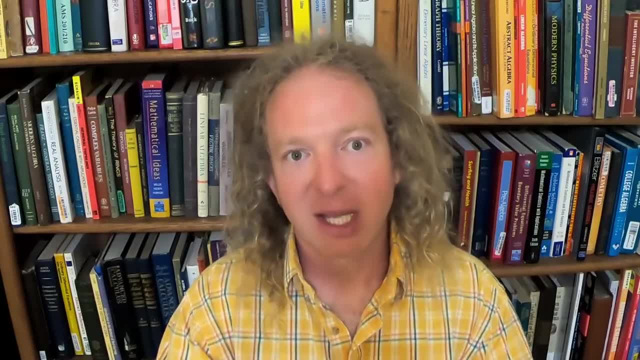 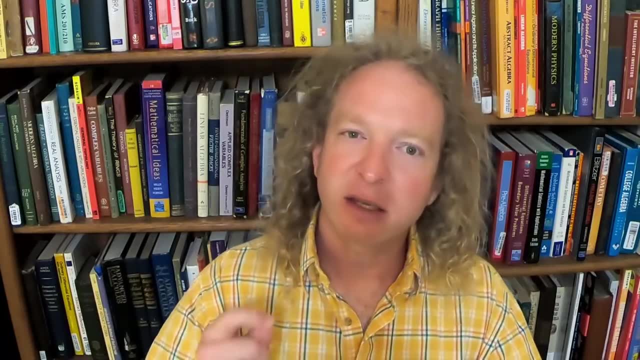 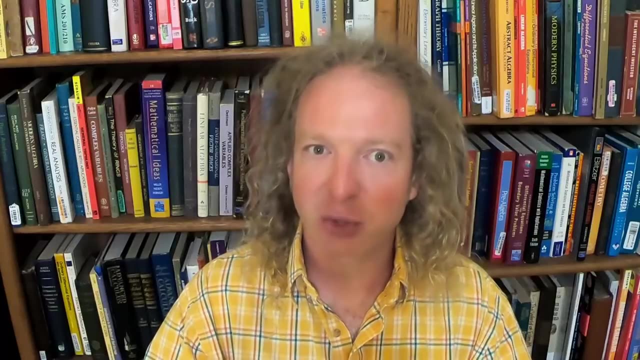 teacher than me, though probably not, but hopefully, you know, by sharing this with you, it will help you in some way. the next thing that you can do is actually something that's a little bit strange, and it's something I've actually. I don't think I've ever talked about this before. it's studying for speed at a speed, yes. 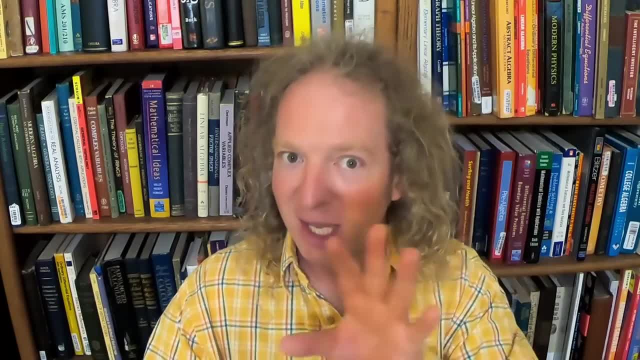 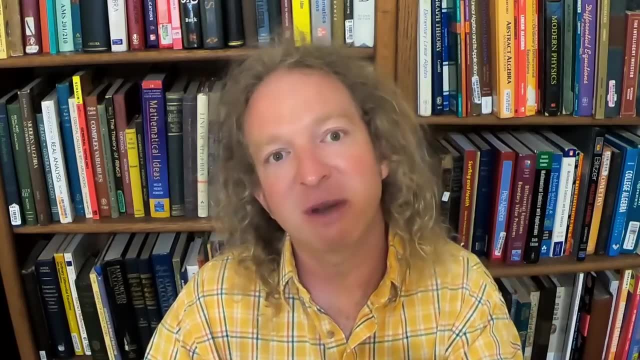 speed. this was something that I was always naturally good at. I was always. There is a negative aspect to being fast and being able to do problems fast. That negative aspect is when you encounter a new topic or a new problem, I tend to want to do it quickly. 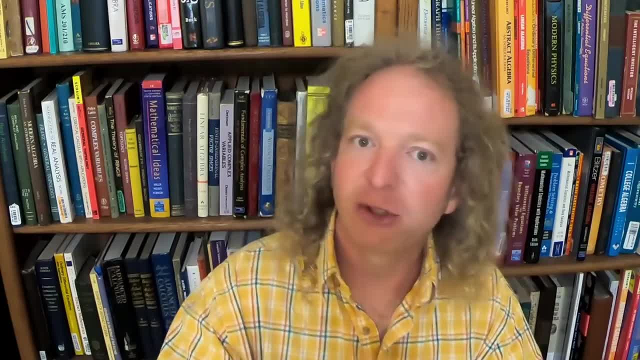 I'm impatient, I'm like, oh, oh, yeah, I can just do it. I should be able to just do it. And then when I get stuck, I'm like, oh, what do I do? So I have to force myself to slow down. 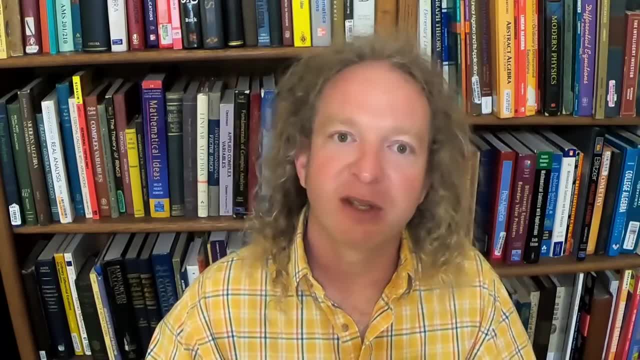 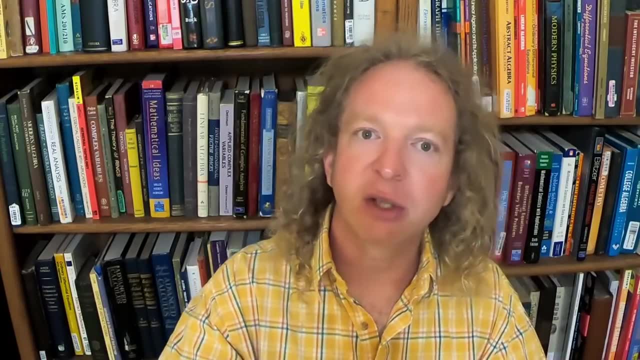 So, on a test for test taking purposes, speed is your friend, So to study for speed, what you do is you make sure that you can actually redo all of the homework problems and all of the examples from the videos or the live lecture that you 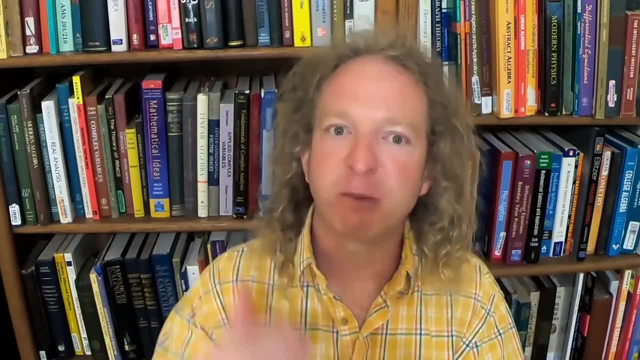 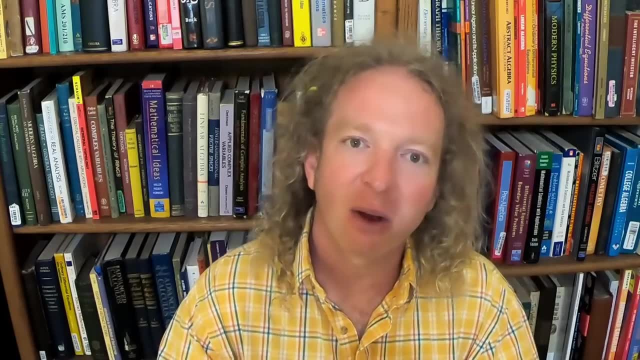 have quickly and correctly Work on speed, And the reason speed is important is because you're taking a time test Now. you might not agree with that. You might say, hey, you know well, I should be able to have more time. 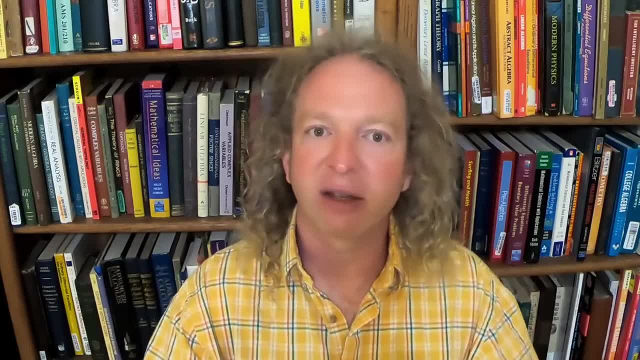 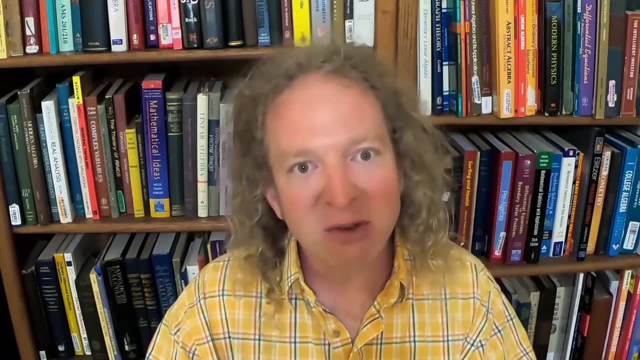 If I had more time I'd be okay. I'm a little bit slow. That is not the reality of life. That is just not how it works. You can't change that. I can't change that. But what you can do is change what you can. 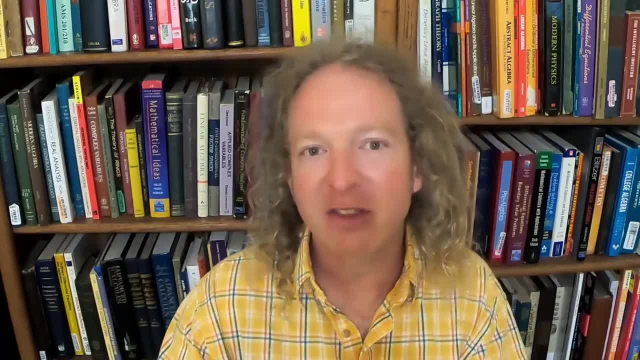 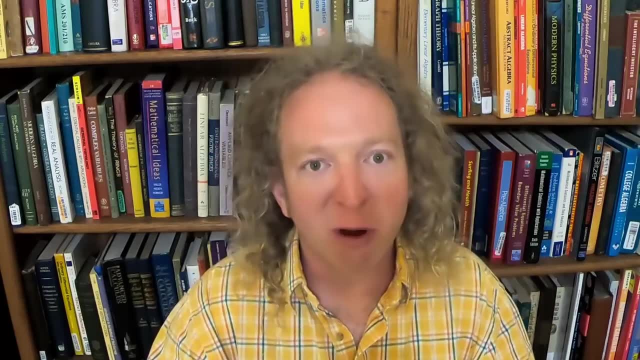 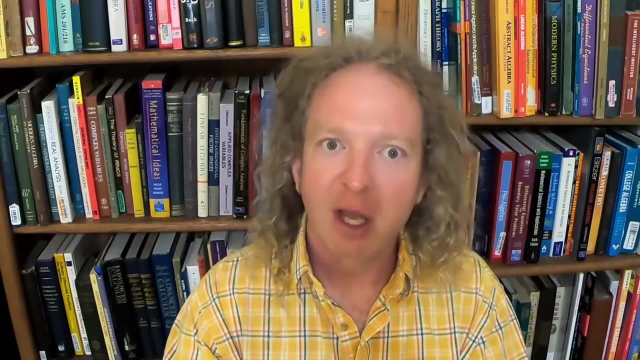 And that's yourself right. Make yourself faster. I had this friend in grad school. The guy was brilliant- I mean, I just got goosebumps So smart. And he was the opposite of me. He was what I like to call a careful thinker. 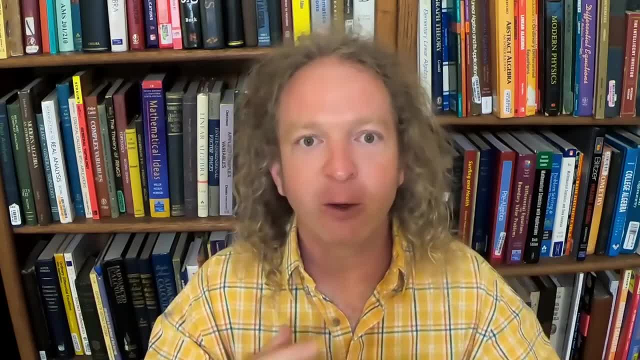 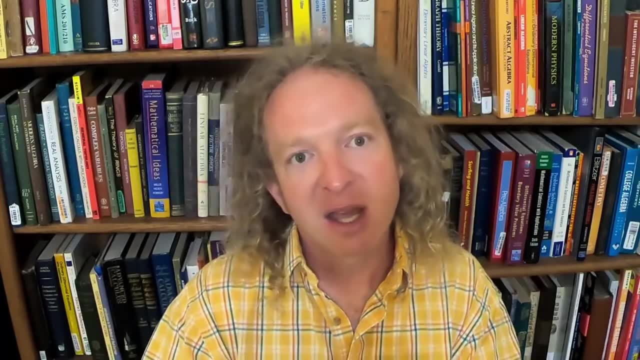 He was able to think slowly and work out really difficult problems in just like beautiful ways, And whenever I work with him I would learn from him, because I realized that I was much faster than him. I would jump into: oh, we could do it like this. 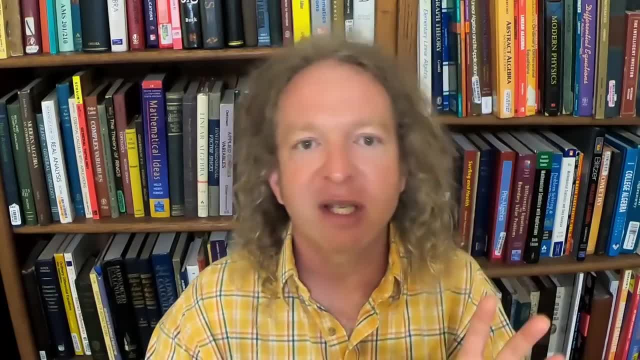 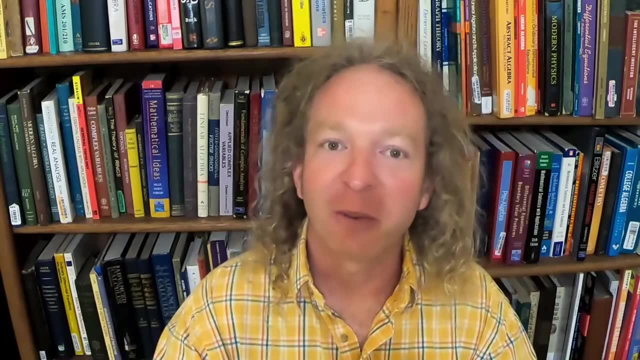 Just choose your epsilon to be this And I would just blow through it, Whereas he had this like well, let's just take it easy, man, And he would like slow down and go a little bit slower. He actually failed a test in grad school. 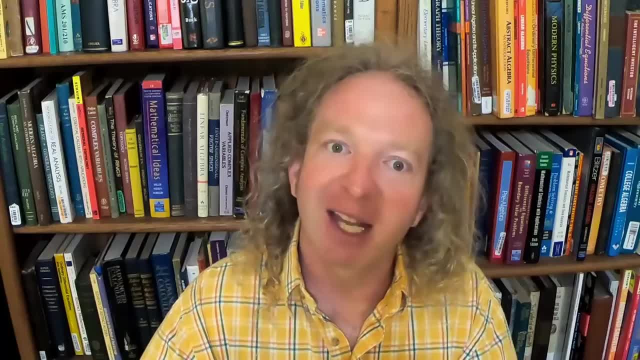 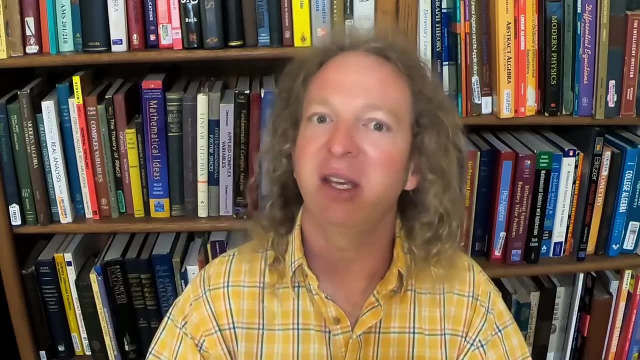 He got like a 40% on a test And he actually came back from that and got an A plus in the class because he was able to work on speed. So speed is important. It is a reality of test taking. So when you're ready for the test, go back and start working on speed. 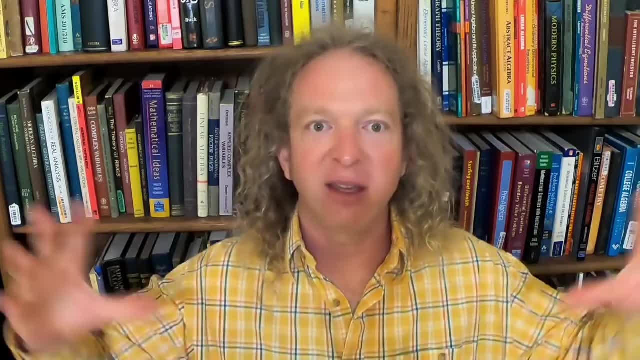 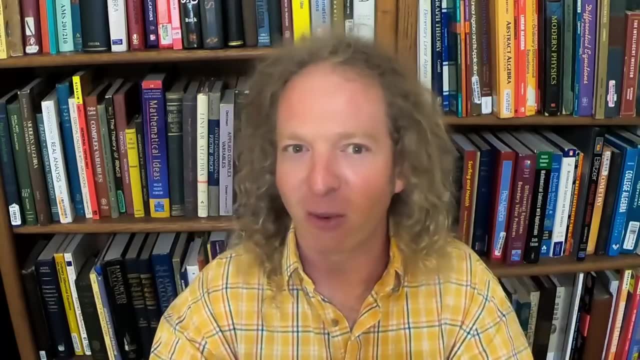 Start doing things fast. This last one is like the- I don't even know the word- the ultimate, maybe it's nirvana. If you reach this, you've reached nirvana. I think I'm using the right word, Maybe not. 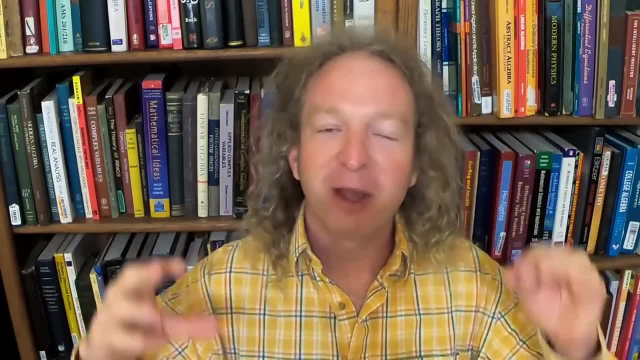 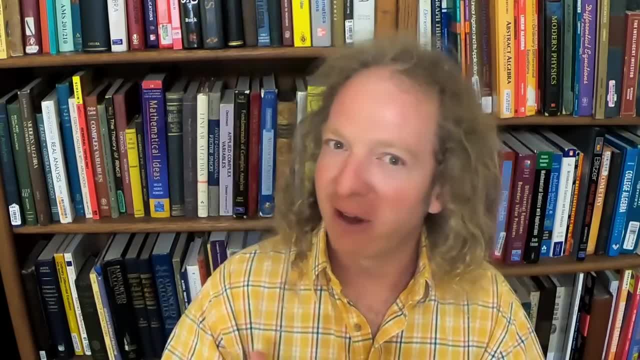 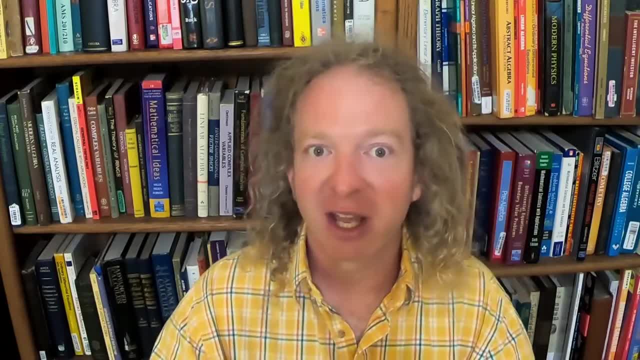 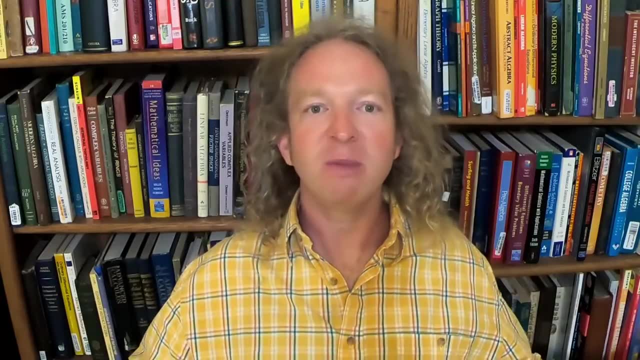 able to reach this stage many times, But I have reached it, And I got this idea from a friend I used to have, because we would all be studying the day before the test and he would be ready for the test. He would just be sitting back and say, hey, what are you doing, man? 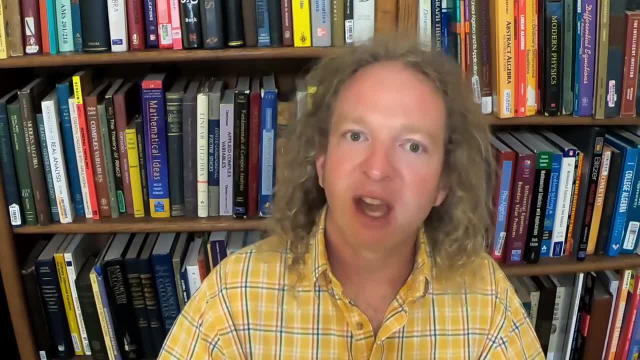 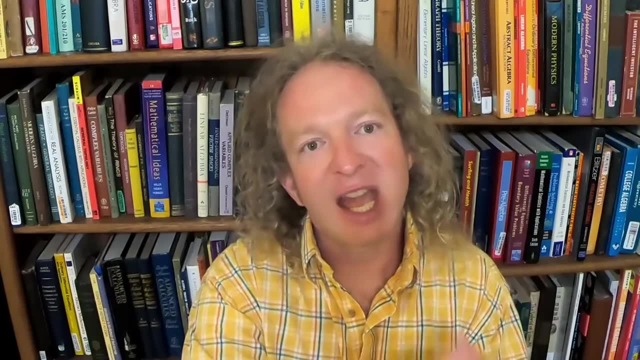 It's like: oh, I'm just going to watch some movies and play some video games and going out with my girlfriend. The test was the next day, But he was done, He was ready, So he would study so much that the day before the test he would just relax. I've done that a few times. 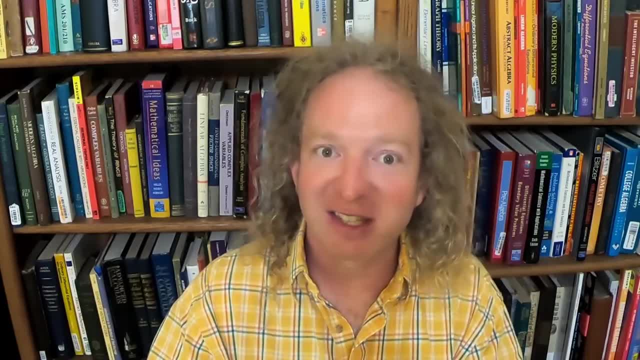 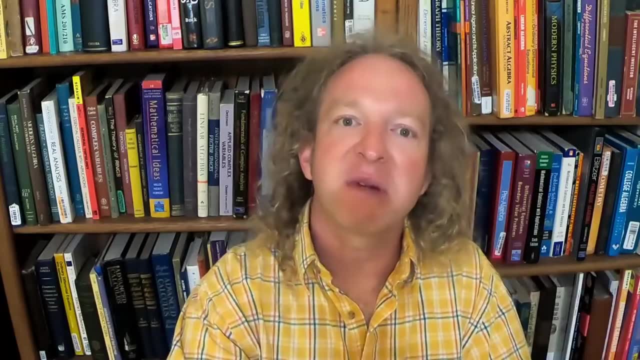 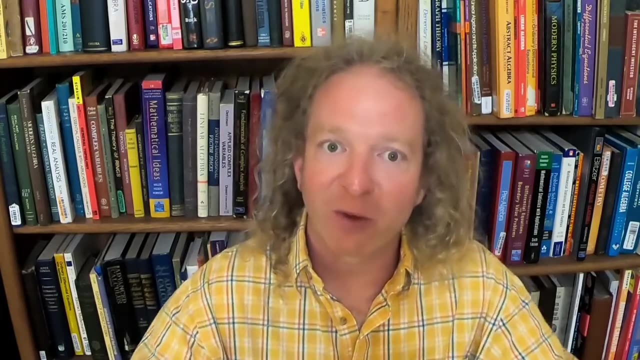 maybe four or five times in my life, and let me tell you, on those tests I have done really well. there's something about like studying a lot and being prepared ahead of time and then just relaxing the day before the test. now, on the day of the test, you should still look everything over. just glance it over, don't.